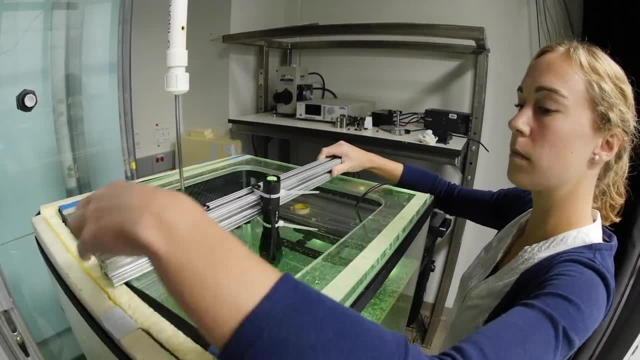 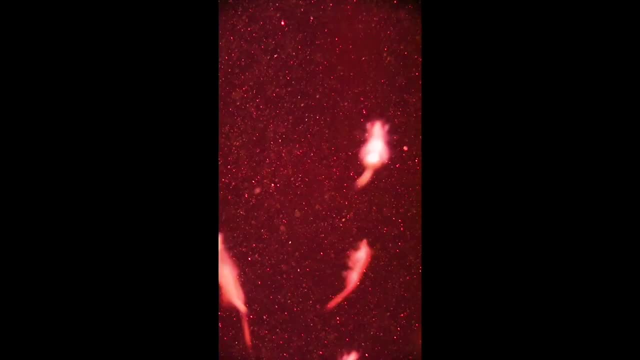 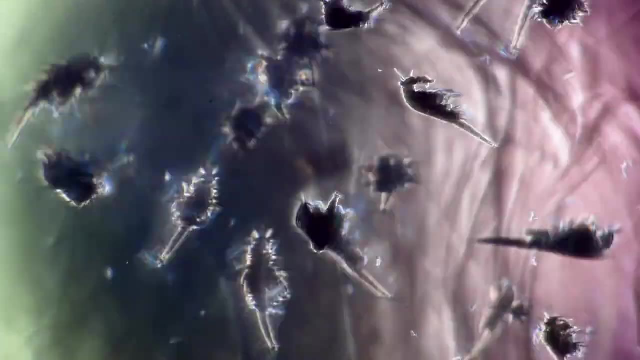 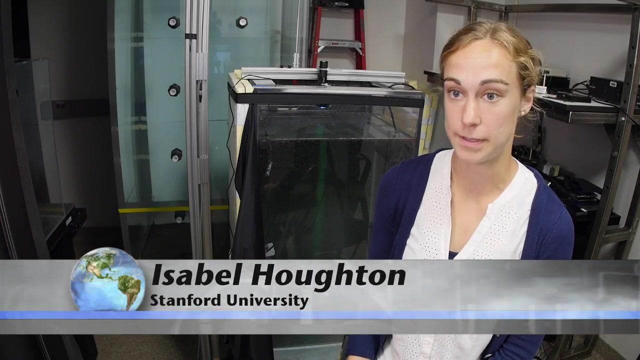 Lights, camera action. Welcome to the magic of the movies. These aren't special effects. These are real images of brine shrimp undergoing what's called a vertical migration. So we have a tank of brine shrimp. They are representative of marine zooplankton, such as. 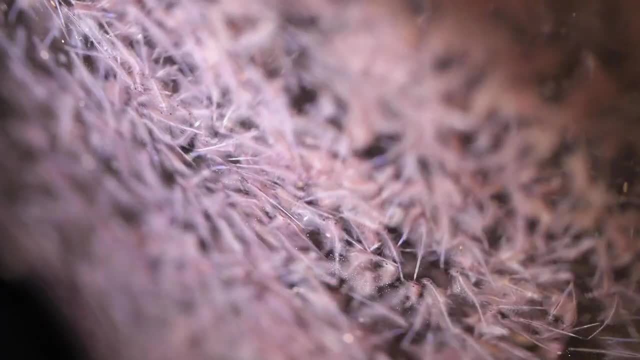 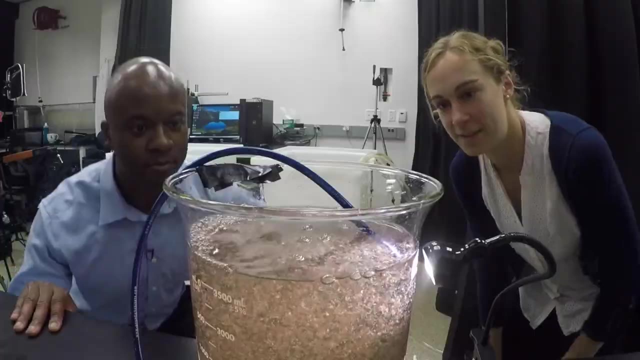 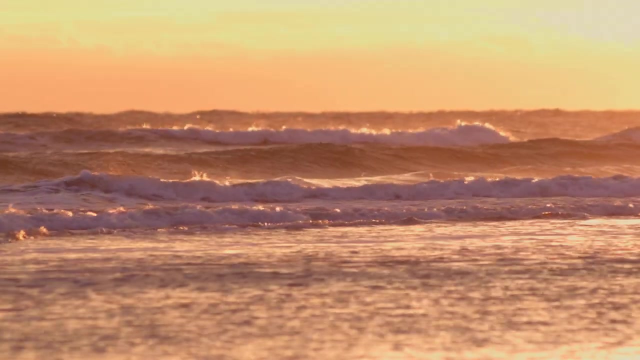 krill in terms of their size and their swimming mode. With support from the National Science Foundation, engineers John Dabiri and Isabel Houghton want to better understand how vertical migrations of tiny marine animals like krill contribute to ocean mixing. We're very interested in how the ocean works because that's going to determine our future. 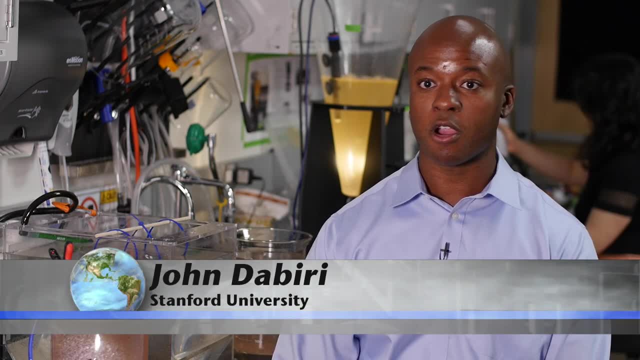 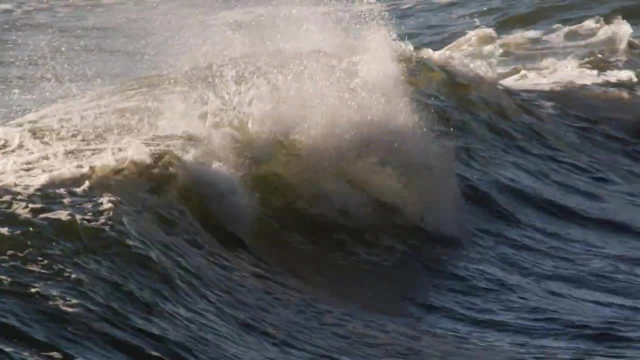 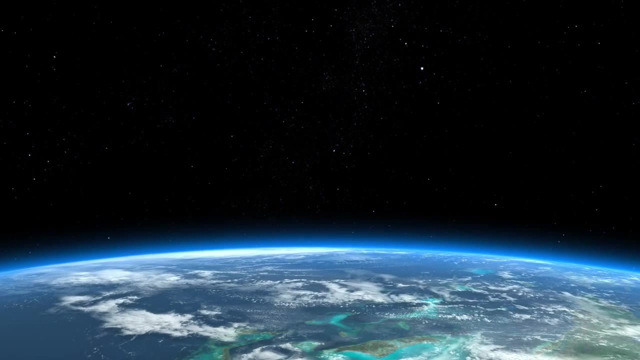 here on earth. The ocean is the primary sink of our carbon emissions. It provides fish for a lot of coastal communities, really for the entire world, And so we're interested in its health and its future. Scientists have long chalked up ocean mixing to winds and tides, but now it looks like 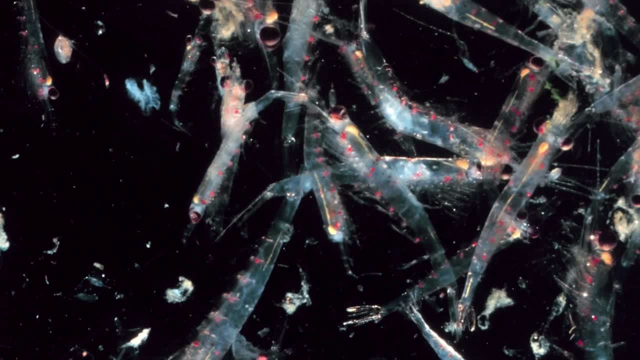 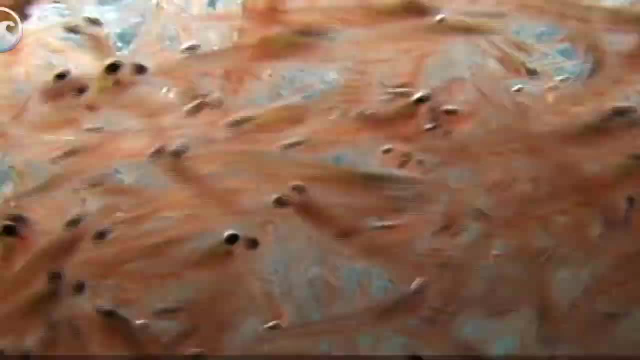 that's not the whole story. Oceans are teeming with shrimp-like krill. They're the base of the marine food chain. Every night, they migrate in giant swarms to the surface to feed. When you have millions of these organisms doing that, you're not going to be able to get them to the 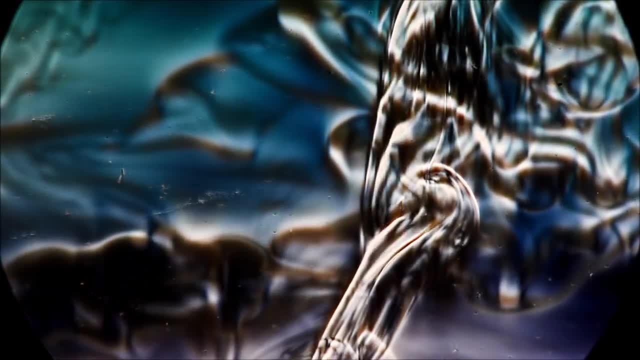 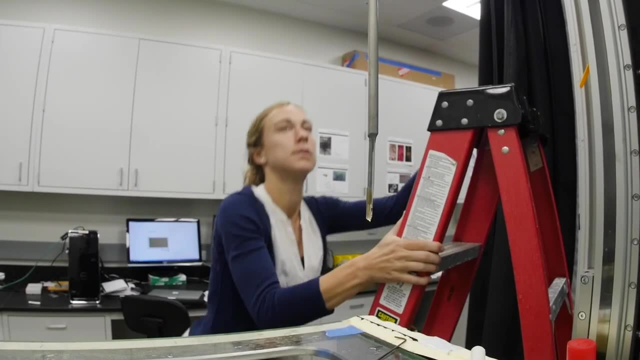 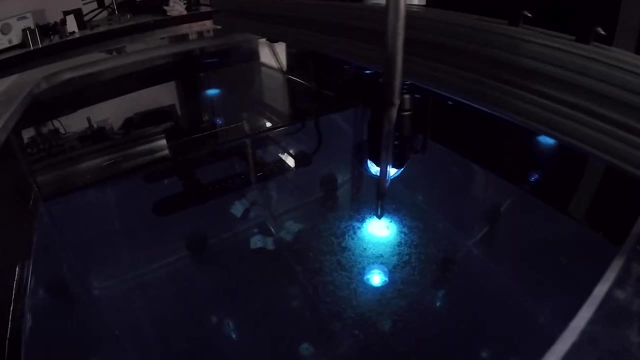 bottom of the ocean. We thought there was the possibility that that downward motion of the water might start to add up almost like a stampede that occurs at the end of each day. In the lab they recreate the vertical migrations using sensors and high-speed cameras to follow what 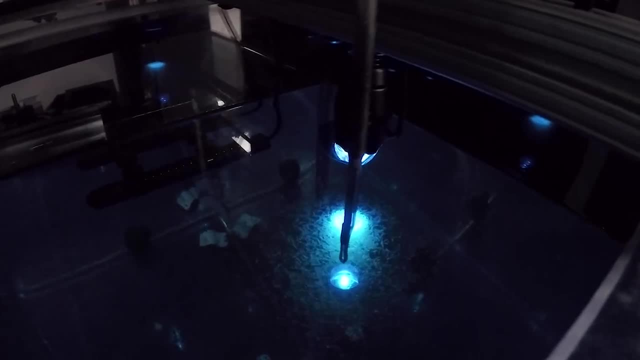 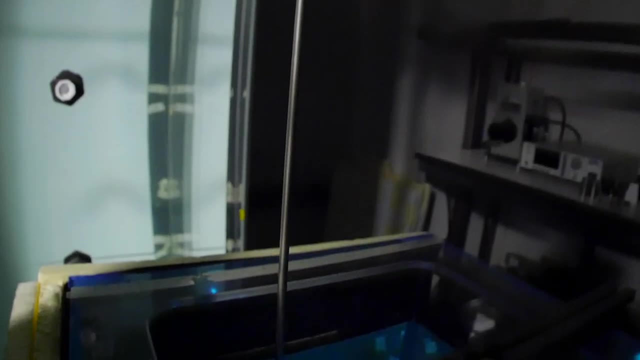 happens as the shrimp swim through different concentrations of salt water. We can actually do laboratory experiments with them to really fully understand the fluid dynamics of what's occurring when you have a migration of salt water. We're going to be able to do a lot of. 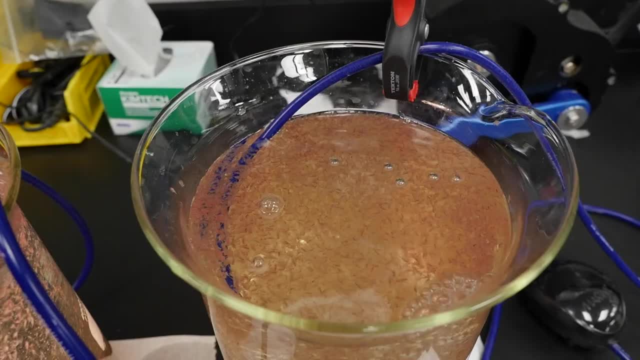 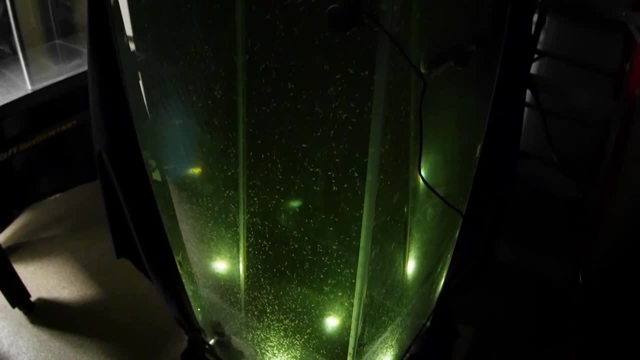 this. We're going to have a swarm through a stratified water column. Brine shrimp are photo-tactic, meaning they'll swim toward light. That allows us to use light sources such as lasers or LEDs to control their motion. Their experiments show that all that kicking really does contribute. 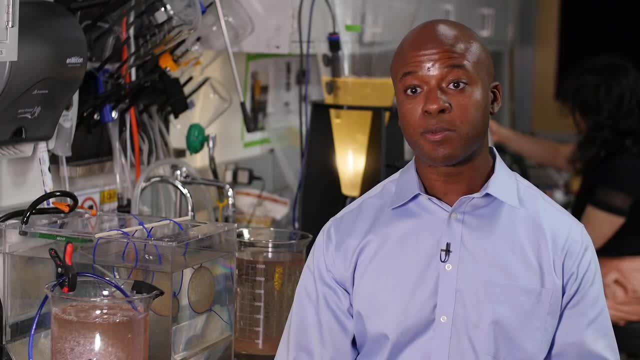 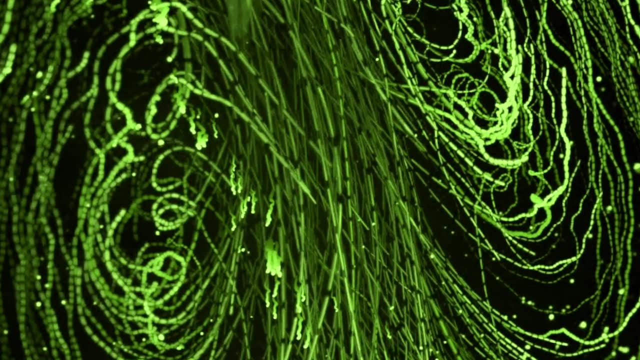 to some serious churn in the water. So we found, surprisingly, that these small animals can have an enormous impact on the mixing of the water column and that they can also create eddies in the water column that are much larger than their ears. We're going to be able to do a lot of this. We're going.